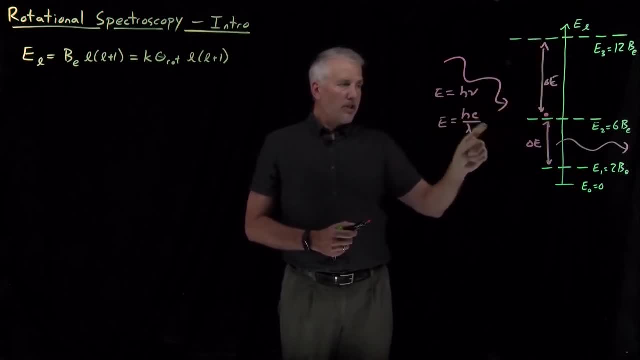 the energies we can calculate the differences between the states, And those differences tell us something about the types of light that can be either absorbed or emitted by molecules that behave as rigid rotors. So first let's take a look at these energy differences, So we know. 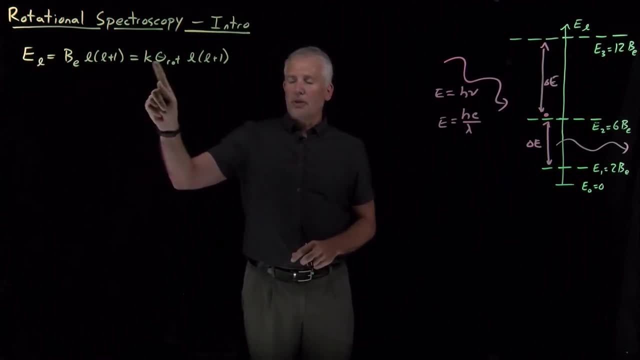 when we've written down the energy differences. we know that the energy differences between the states are. when we've written down the energy differences between the states are in the energies, either in terms of a rotational constant, or sometimes, if we prefer a rotational constant, or sometimes if we prefer a rotational temperature, The energy levels are either zero or 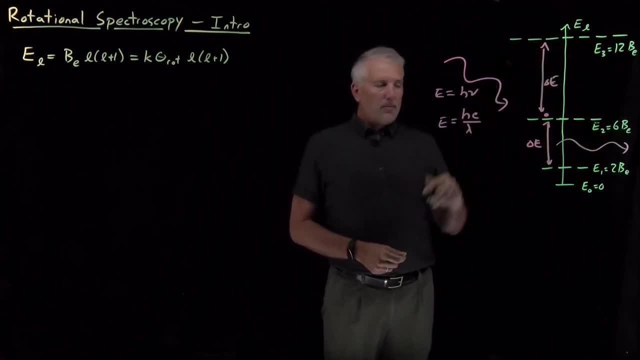 twice the rotational constant, or six times, or 12 times, or 20 times and so on. So the gaps between those energy levels. this delta E would be twice the rotational constant: 2BE minus zero. This one would be: 6BE minus 2BE, is four. This one, 12 minus six, is six. So each of these energy differences, 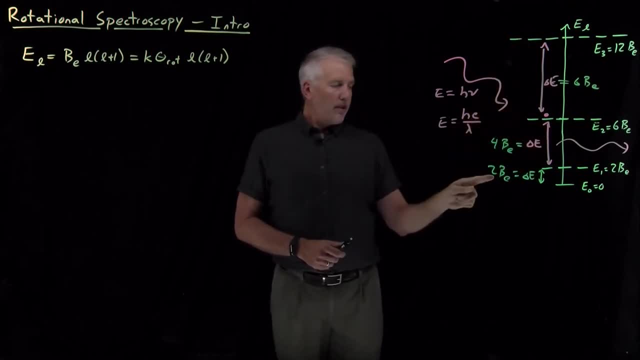 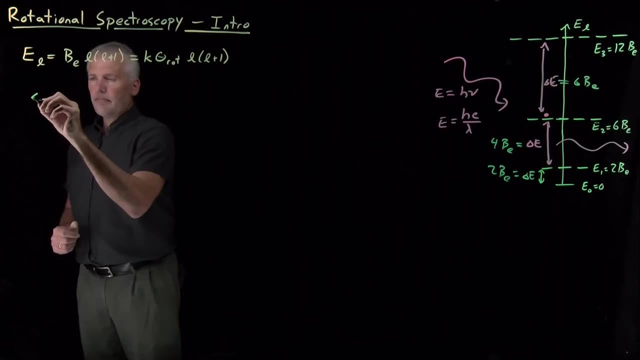 is different. They get larger as they go up. The size of those gaps goes from two to four to six, The next one will be eight, and so on And in general. so if I want to know, let's say for the L to L plus. 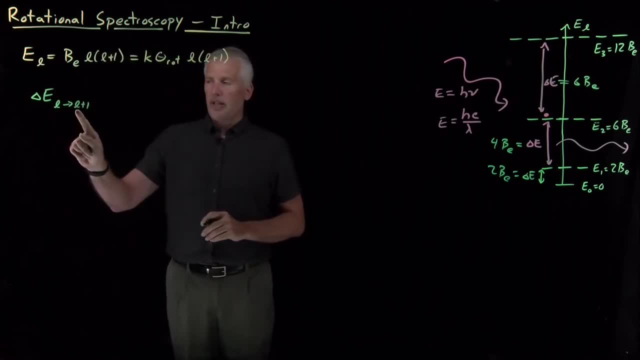 one transition: the gap between the ELF energy level and the L plus one energy level. that's going to be the energy of the upper level minus the energy of the lower level. We have an expression that tells us how to calculate each of those. 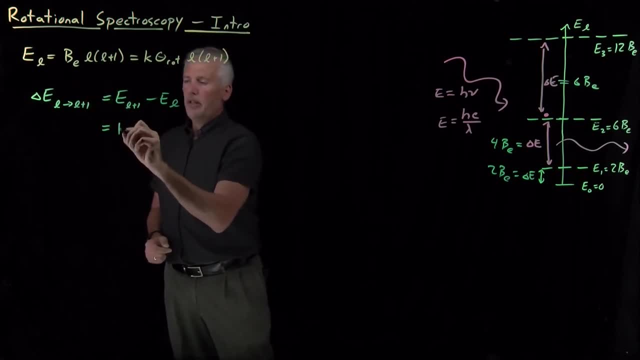 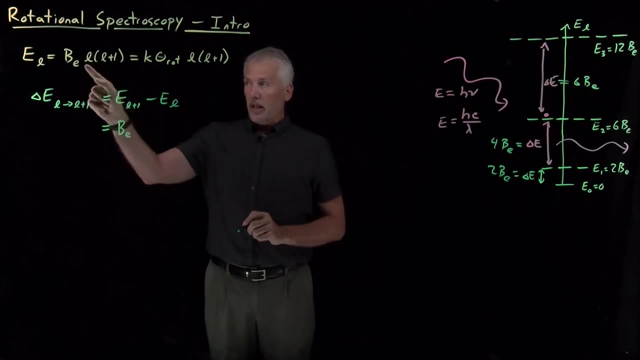 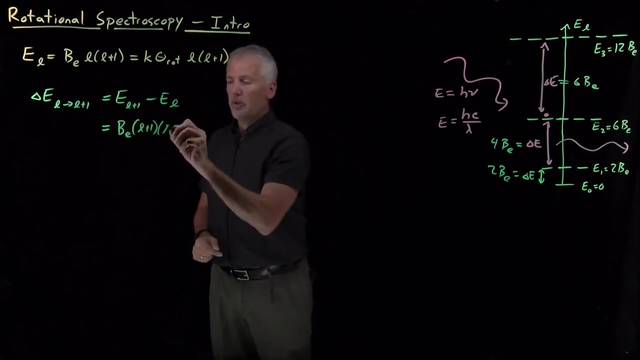 So the L plus 1 level has an energy of a rotational constant, not times L and L plus 1, but when I am asking about the L plus 1th level, L has the value L plus 1.. And L plus 1 now is 1 higher, so that's L plus 2.. 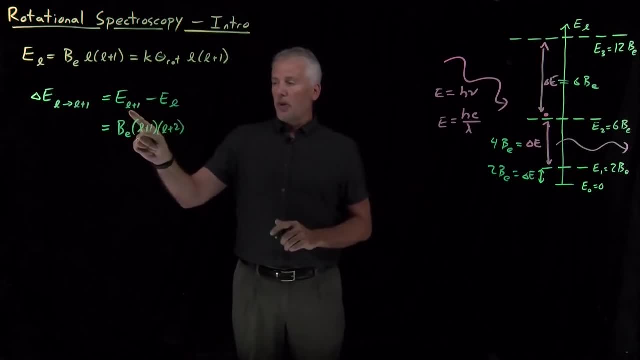 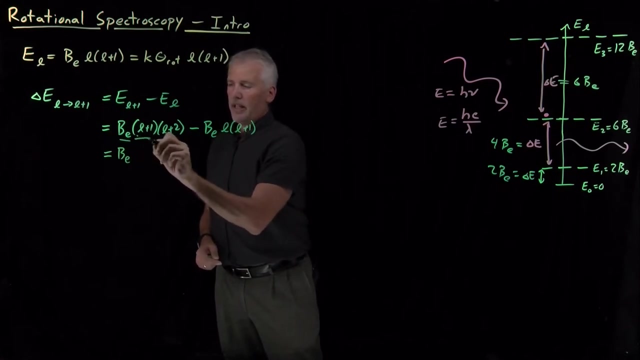 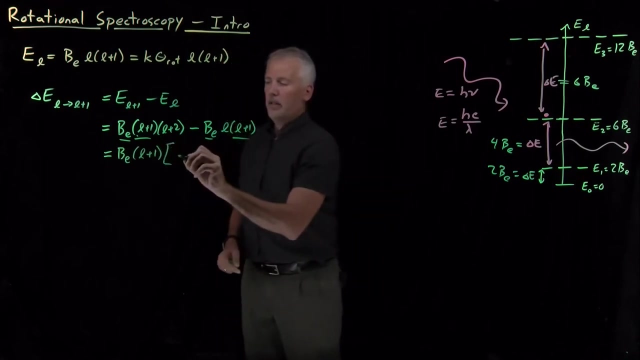 So that's the energy of level L plus 1.. Level L is still L times L plus 1.. So that simplifies a bit. So both of these terms have a BE and an L plus 1 in them, And what's not included out front, I have an L plus 2 minus an L. 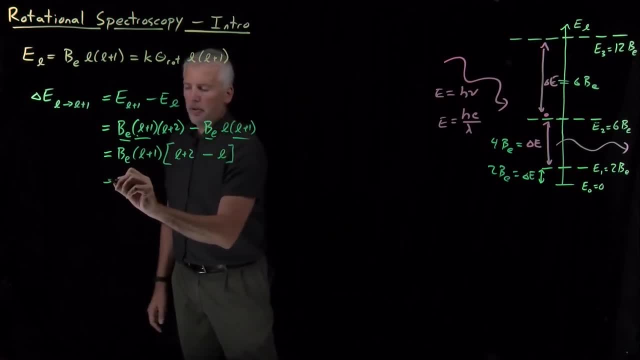 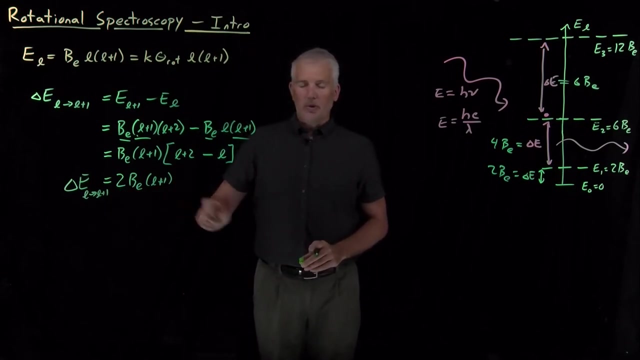 And the Ls cancel, leaving me with just a 2, and I can say, okay, That the gap, this energy level difference, in going from L to L plus 1, is twice the rotational constant times L plus 1.. So it's no coincidence that these gaps were going up as even numbers. 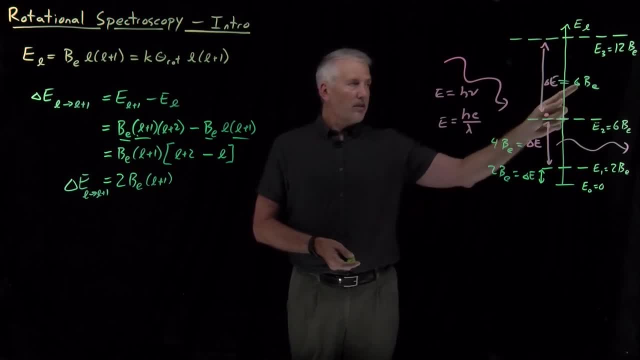 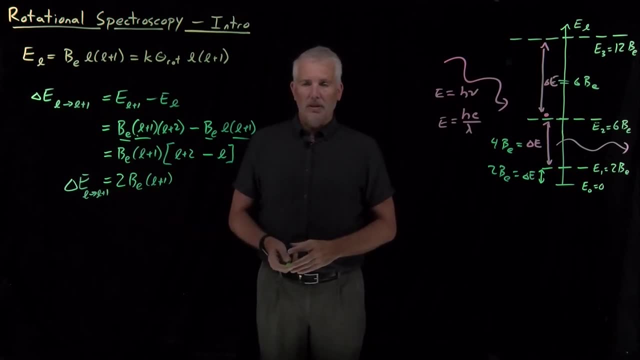 twice the rotational constant, four times the rotational constant, six times the rotational constant. That pattern will continue, continue going up as even numbers multiplying the rotational constant. So now, if we want to know that, for some reason, the gap between the 21st 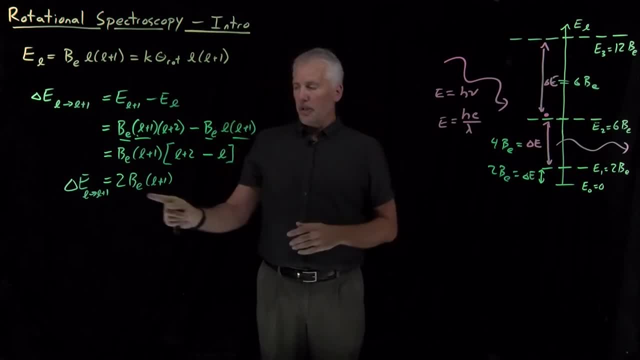 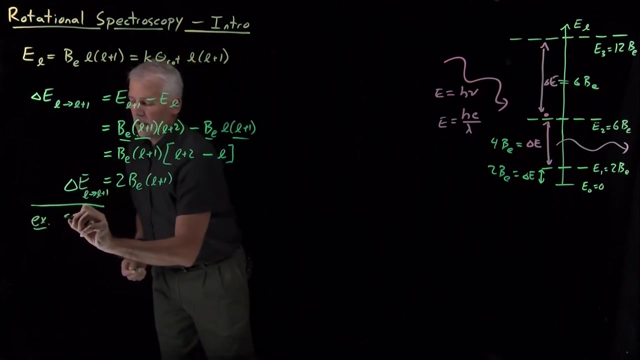 and the 22nd energy level is just going to be twice the rotational constant times 22, the upper level. So that's enough to tell us what the gaps are. We can let's go ahead and use some actual numbers. So let's ask again about the carbon monoxide molecule. 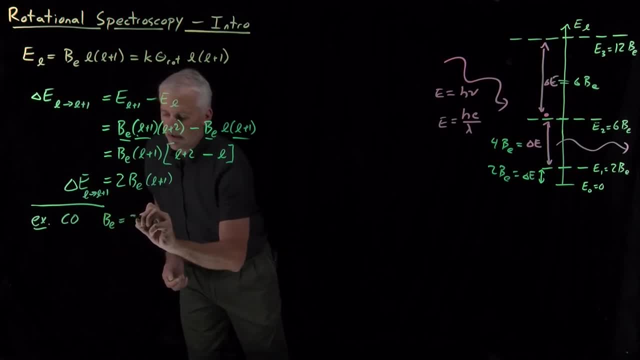 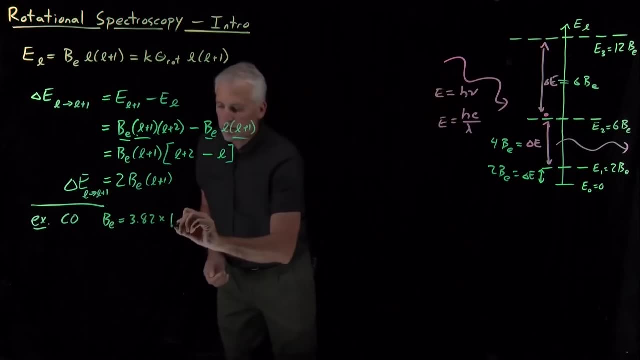 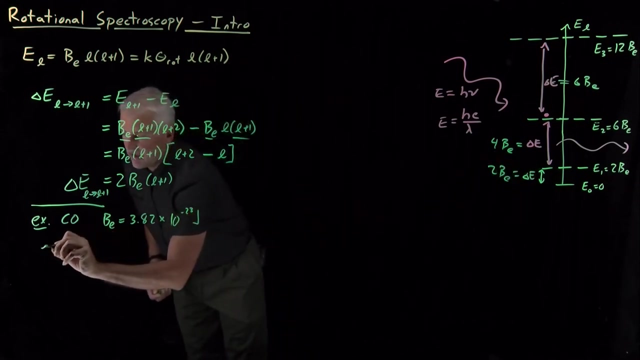 for which we know, or I'll tell you the rotational constant: 3.82 times times 10 to the minus 23rd Joules. So we could now calculate. let's go ahead and say: for the L equals 0 to the L equals 1 transition. 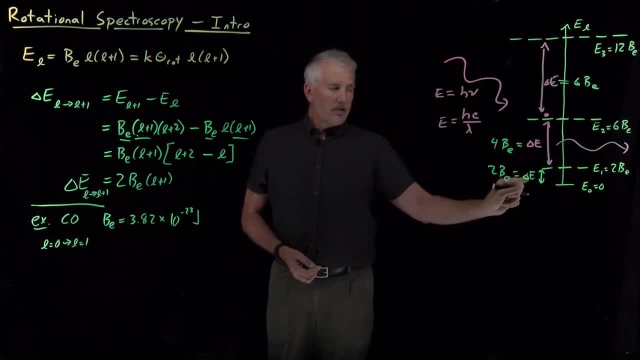 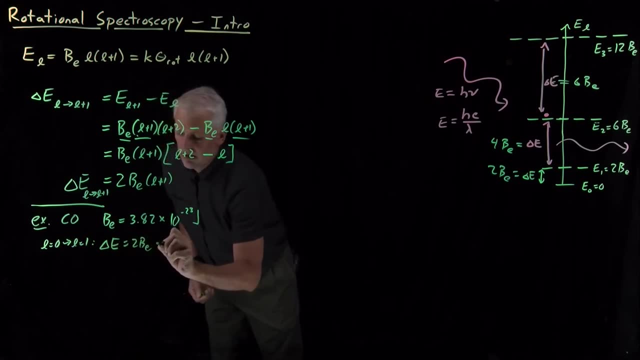 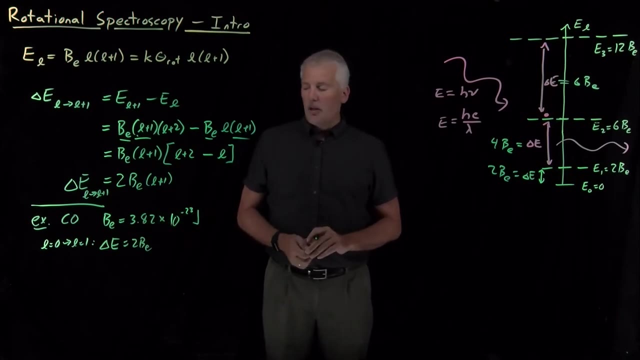 this gap between the levels, so that delta E is going to be twice the rotational constant, which would be twice this number 7.6 times 7 minus 23 Joules. So that's a number in Joules More interesting than knowing how many Joules what the energy level difference is. 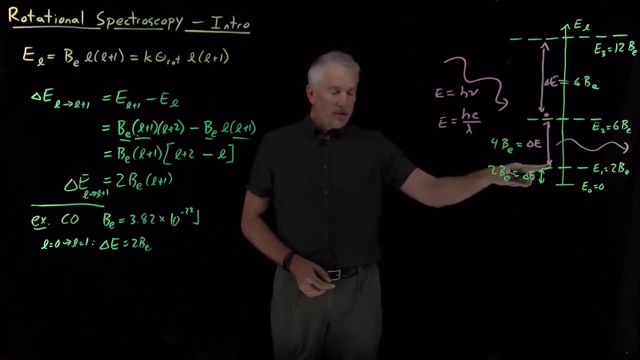 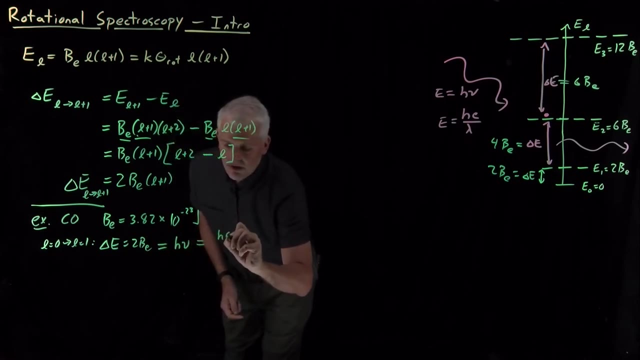 is knowing something about the light required either to induce that transition upwards or the light that's emitted when a molecule falls down from the L equals 1 to the L equals 0 level and a photon gets emitted. So if that energy difference is equal to either H times nu or HC over lambda, 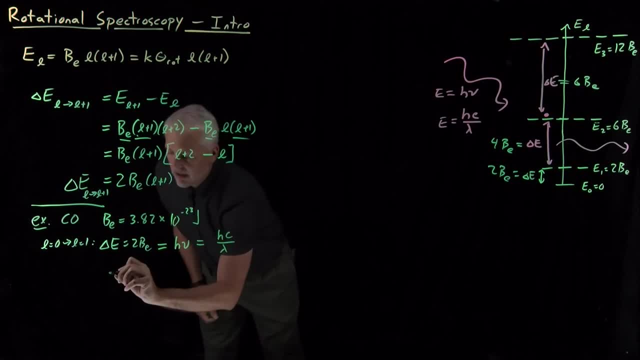 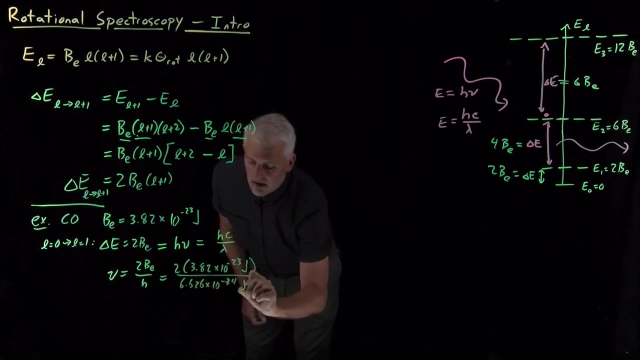 we can ask ourselves: what would that frequency be? The frequency would be rearranging this expression twice: BE over H, So twice this rotational constant divided by Planck's constant. So thinking briefly about units, Joules on top from the rotational constant, cancel the Joules. 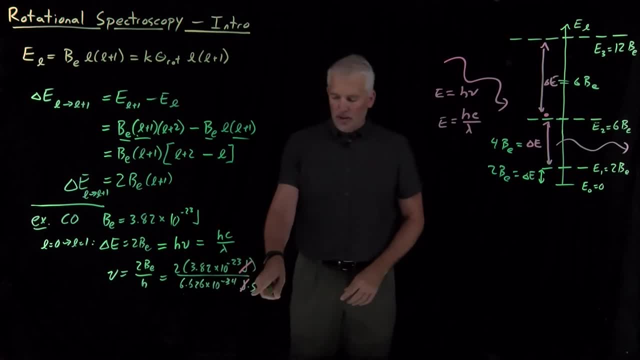 that are hiding inside of Planck's constant. The units leave seconds in the denominator, So the units are going to be 1 over seconds, which is correct for a frequency, And if we do the math, that frequency turns out to be this number. 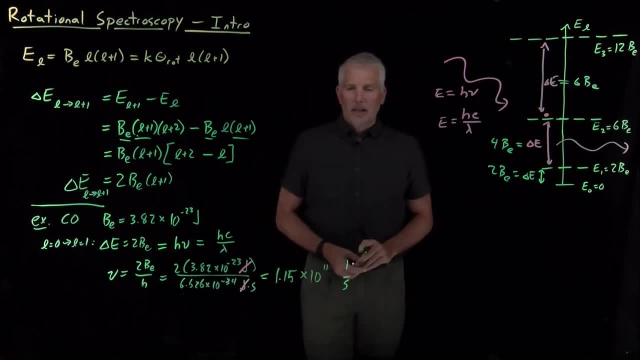 1.15 times 10 to the 11th per second. So the frequency of a photon used to excite this rotational transition from a nonrotating molecule up to a slightly rotating L equals 1 rigid rotor state would be 1 over seconds. 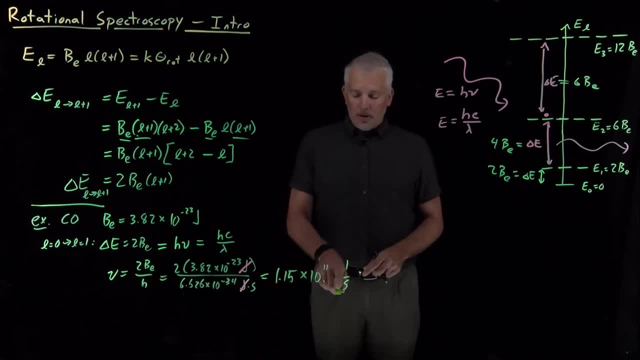 Right would be 1.5 times 10 to the 11th per second. That number perhaps is not terribly intuitive. Let's try instead the wavelength. We might get more information out of knowing what the wavelength of that photon would be. 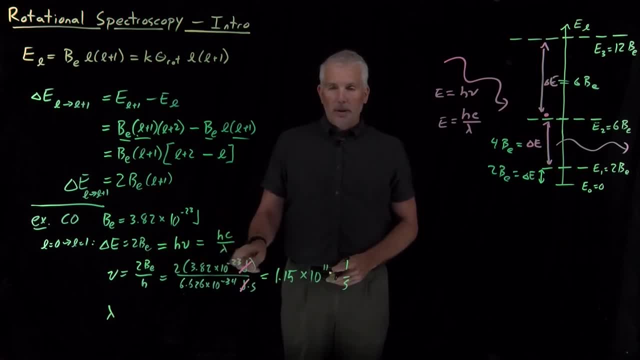 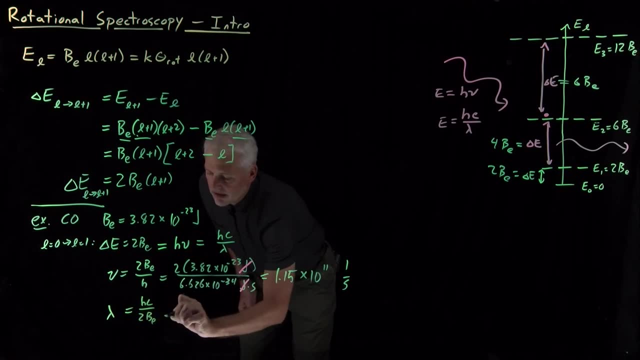 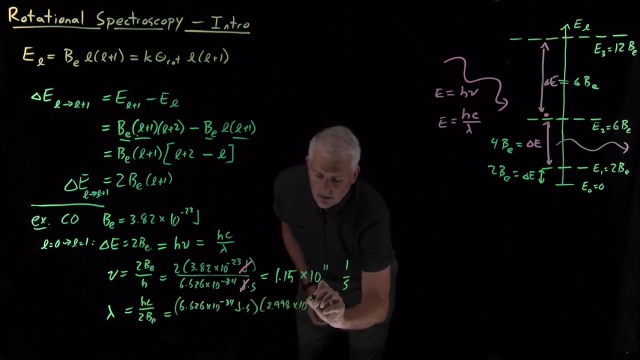 So if I rearrange 2B, equal to HC, over lambda, I'll get: lambda is equal to H times C divided by twice the rotational constant. So again Planck's constant multiplied by the speed of light, 3 times 10 to the 8th meters per second. 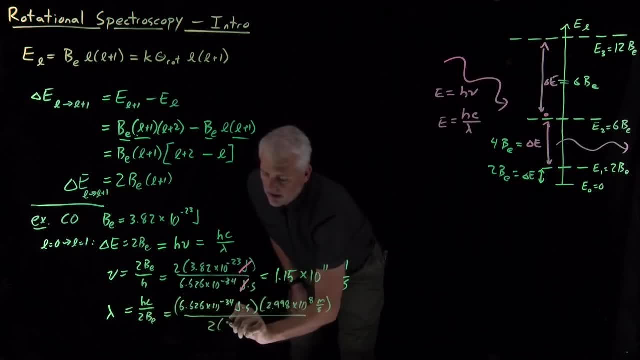 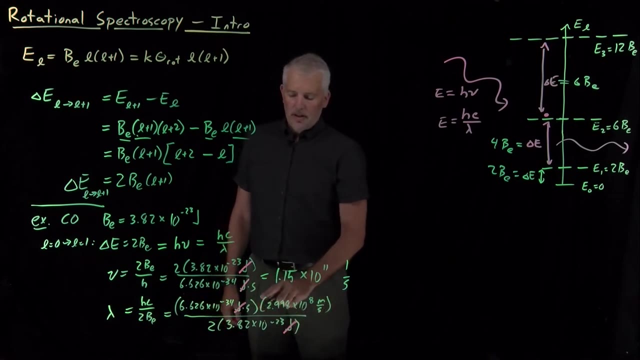 and divide all that by twice the rotational constant, The units. in this case again I've got joules from Planck's constant which cancel joules in the rotational constant. Planck's constant has units of second which cancel one over second in the speed of light. 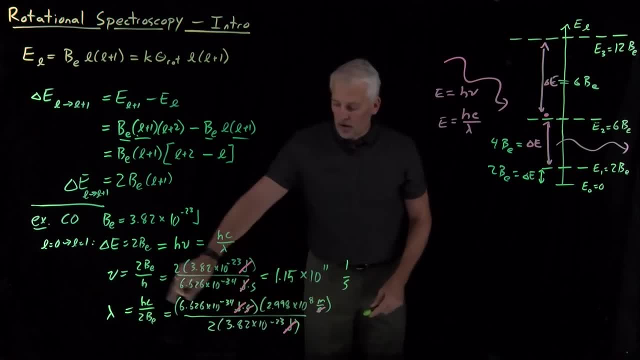 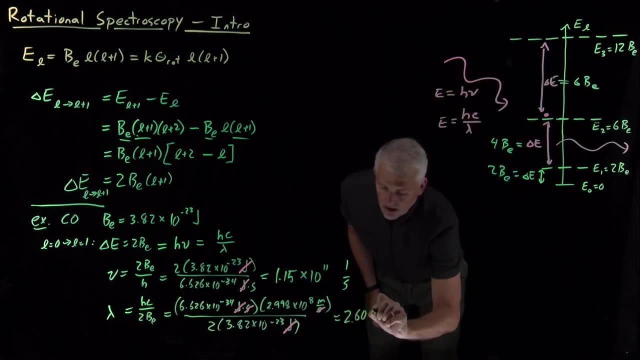 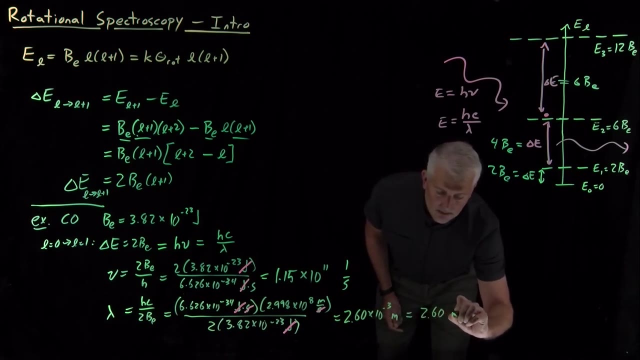 And the units I'm left with are just meters, which is correct for a wavelength. Numerically, that answer turns out to be 2.6 times 10 to the minus three meters or, if we prefer, 2.6 millimeters.